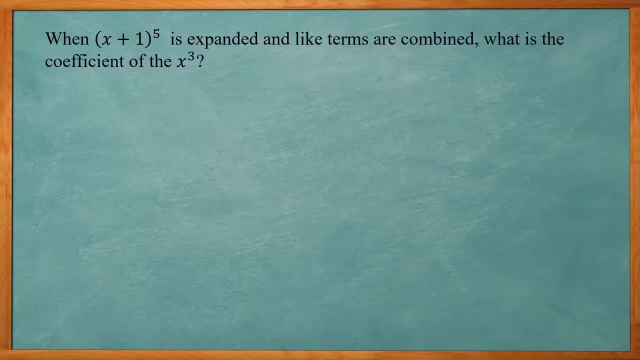 Now you could FOIL this out, but you would need x plus 1 five different times and multiply it out and that would take a long time to do. And problems on an ACT shouldn't take more than one minute, or even two minutes. If it's past that, that's a problem. you should skip and move on to a different problem. 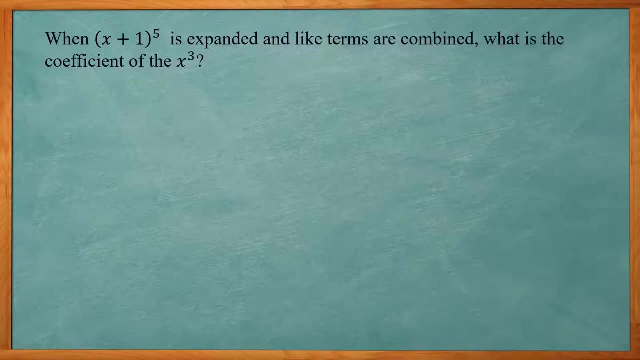 But here we can solve this one fairly quickly using Pascal's Triangle. So Pascal's Triangle is used to find the coefficients of binomials to x power. So here we have x plus 1 to the 5th power. So for the triangle we start out at 1, at the top of the pyramid. 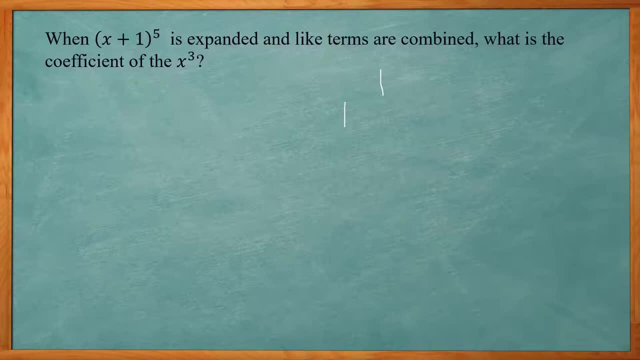 So we do a 1 over here, a 1 over here, then a 1 here. Now in the middle we add the two numbers that are above it: 1 and 1 is 2.. And at the end is 1.. 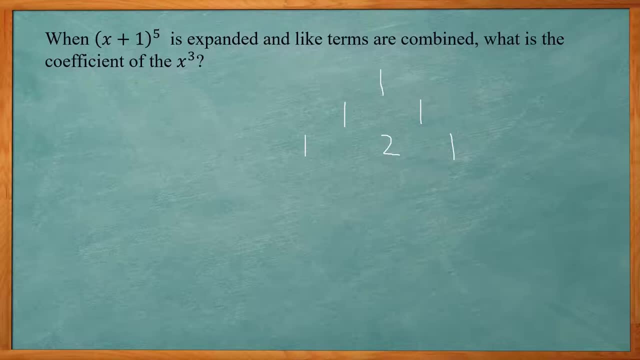 Alright, so again we go to the next level. There will be a 1 here, There will be a 2 here. Then we get a 1 and 2.. We add those together to get 3.. And a 2 and a 1 to get another 3.. 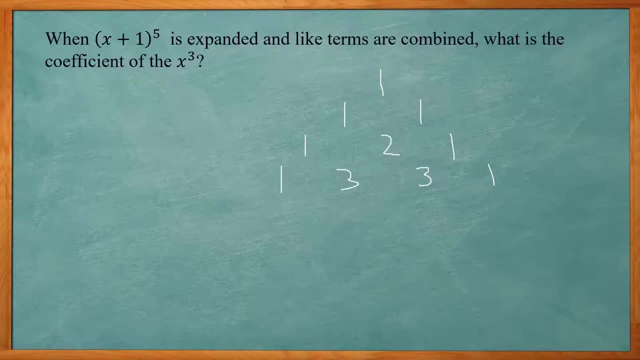 And then the 1 at the end, And the next time we do a 1, here We have a 1 and a 3 to give us 4 that we add up. 3 plus 3 is 6.. 3 plus 1 is 4.. 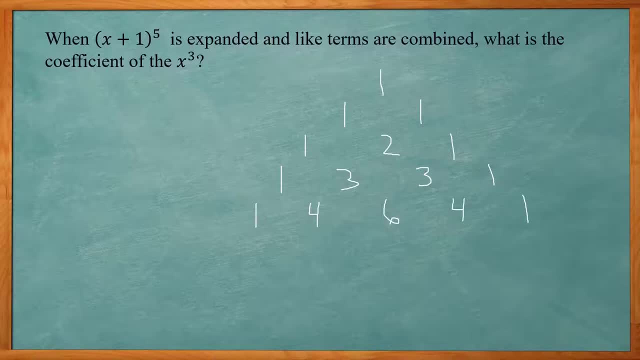 And a 1 at the end. Then we go again. We got a 1 here: 1 plus 4 is 5.. 4 plus 6 is 10.. 6 plus 4 is 10. And 4 plus 1 is 5.. 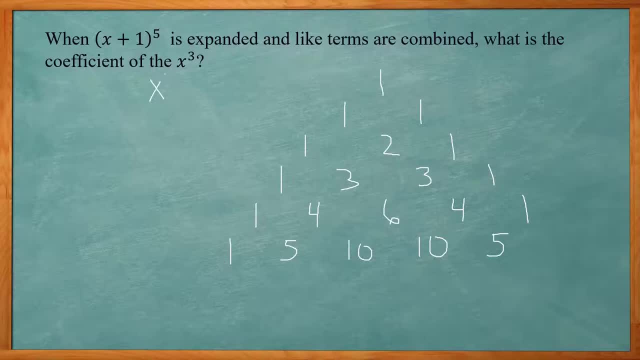 Now, at this top level, this is x to the 0 power And x to the first power, x to the second, x to the third, x to the fourth And x to the fifth. So we have x plus 1 to the fifth power.